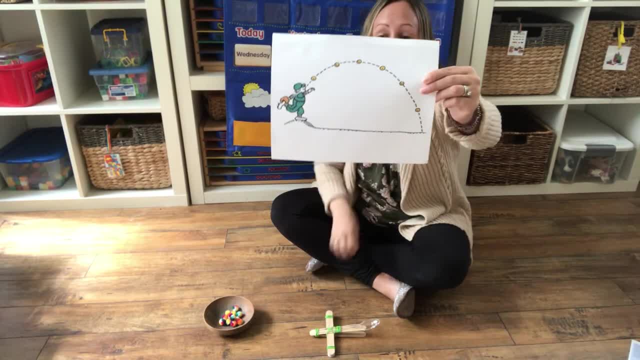 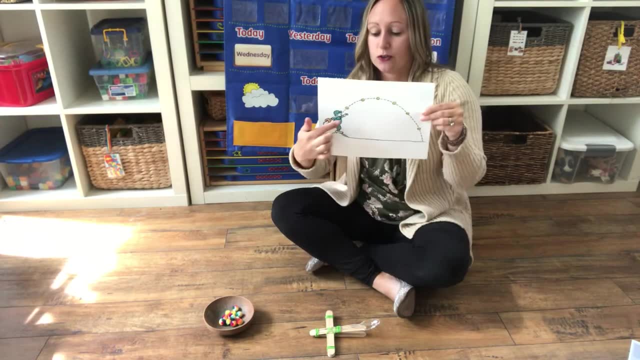 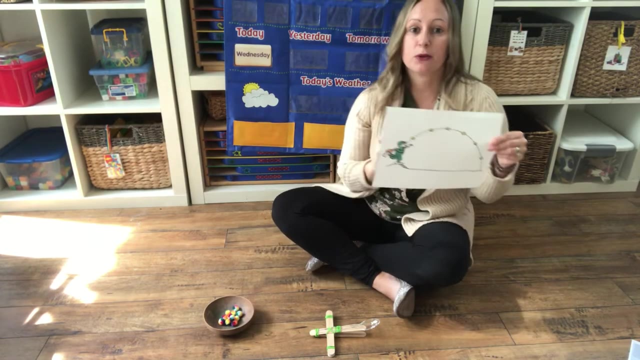 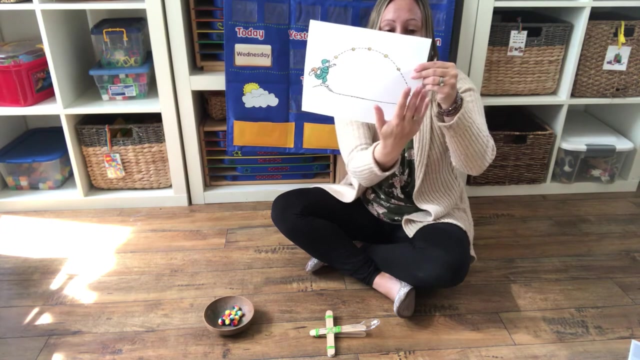 It makes an arc. It makes an arc So there's different forces that are acting on that ball that cause it to move in that kind of a motion. So the hand holding the ball makes the ball move Right, Makes it move, And there is gravity that is pulling down on the ball and the air friction is slowing it down. 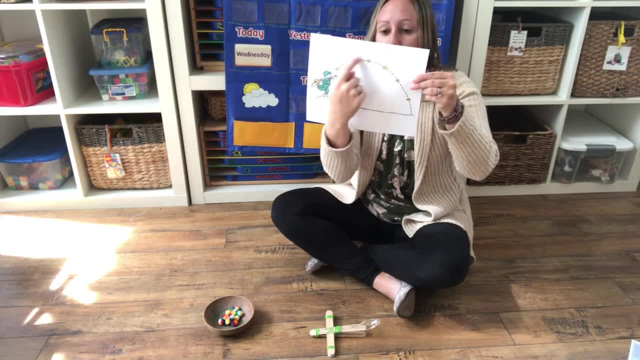 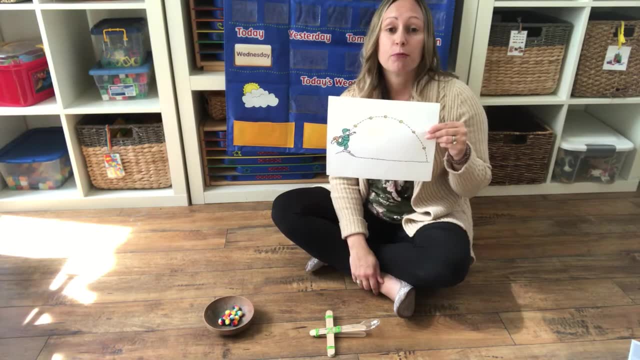 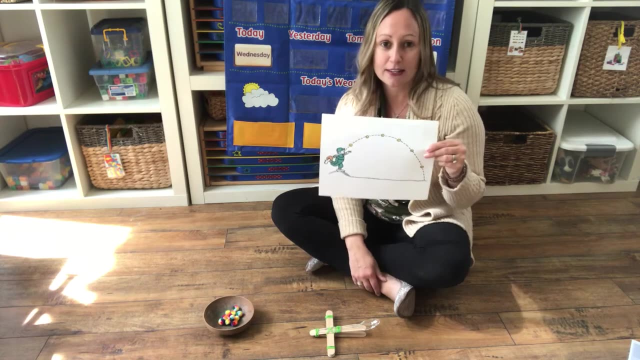 So this motion that we are learning about looks like a rainbow. It's an arc. There's a special science name for it: It is called projectile motion. And now, if any of your moms or dads are listening, they might think of something else when I say that word, Because we sometimes think about that when little 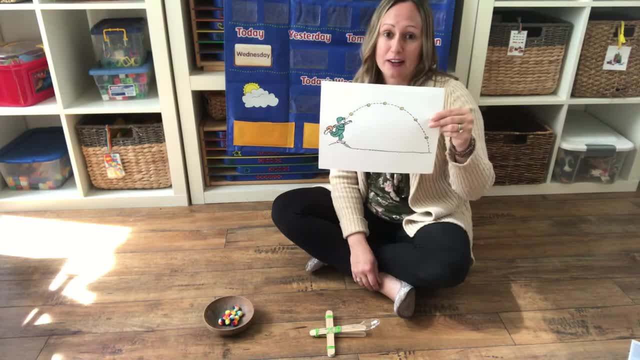 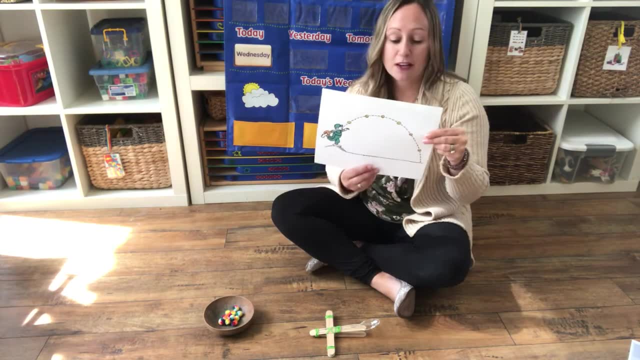 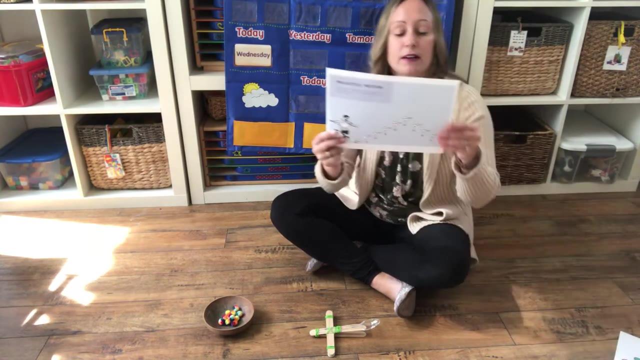 kids are sick. But for today we are going to be talking about how that works in sports. How that works in sports And we're going to have some fun with it. So think about that: when you throw something, it makes that arc. Or if you kick something, like with this soccer. 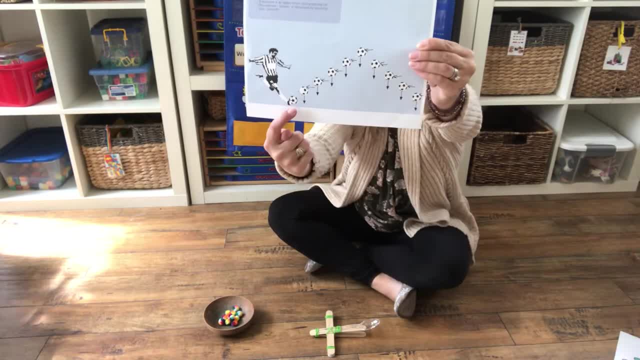 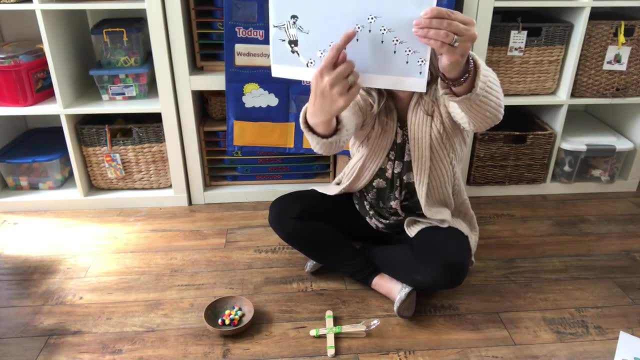 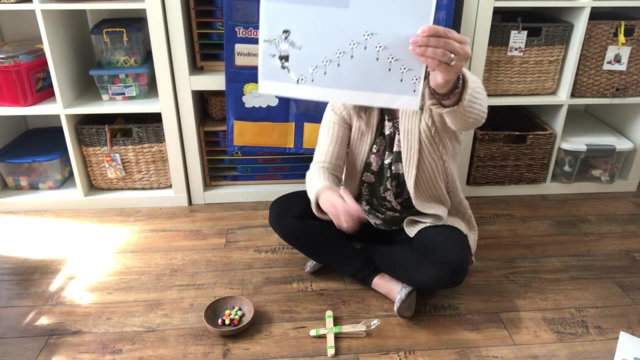 ball. you can see that the person's foot kicks it. It goes up and then down And there's arrows on this one showing it's being pulled down by gravity, by the magnet that's inside it, And it's being pulled down by gravity And it's being slowed down by the friction and 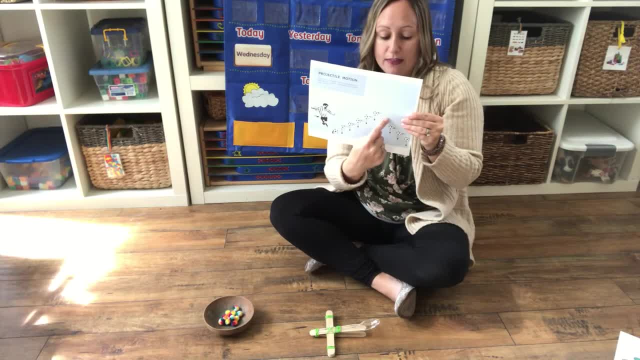 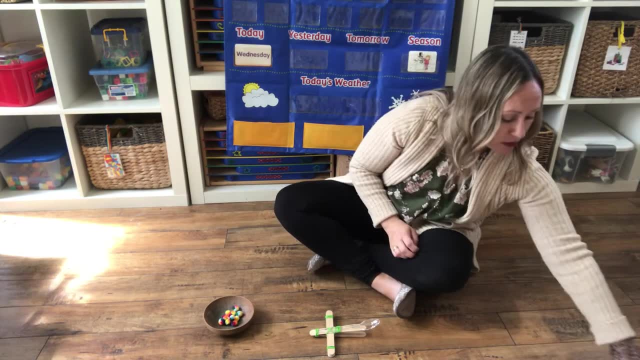 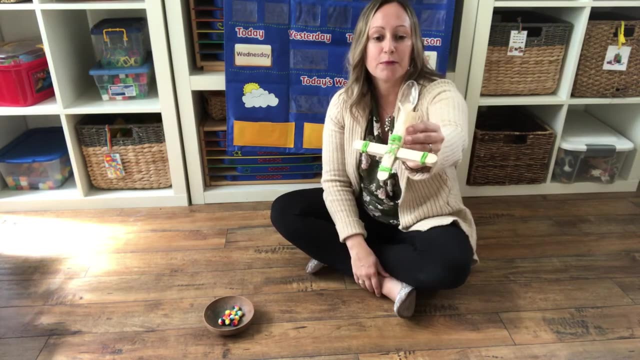 air. So we kick it up and then it comes down. It makes an arc just like when we're throwing or hitting a ball. So a really fun way to test this out is by making a catapult, And I have on my website a bunch of different kinds of catapults you can make. If you don't. 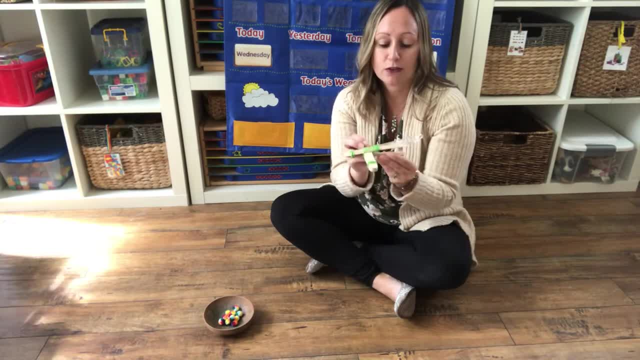 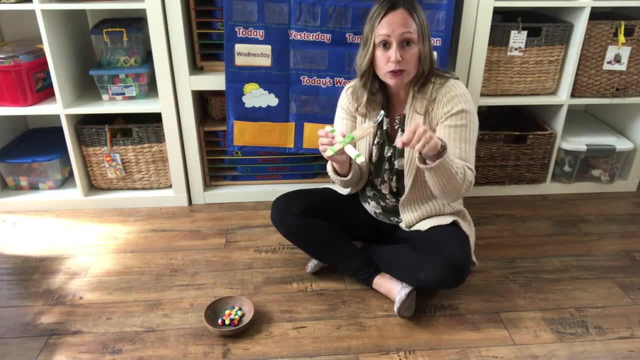 happen to have popsicle sticks In your house, you can do it with just like a paper towel roll or a toilet paper roll. Or if you don't even have that, you can get some paper and just roll it up nice and tight and attach a spoon on there so you can make a catapult.